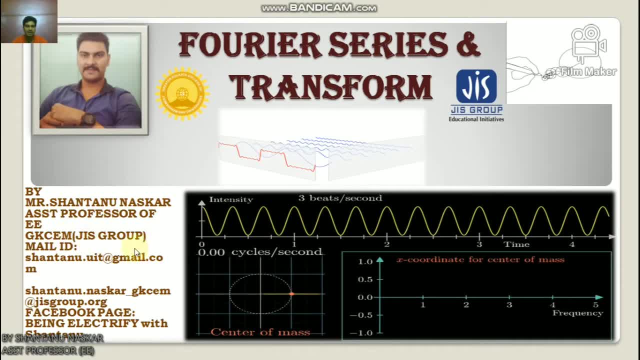 Department GKCMJIS group, and my mail id is santanuuit at the rate of gmailcom and santanunosgore gkcm at the rate of gisgrouporg. and this is my facebook page being electrified with Santanu. You can get all the lecture in my facebook page and also in my youtube channel. 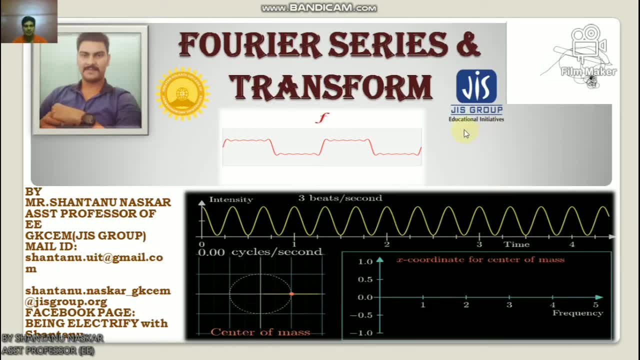 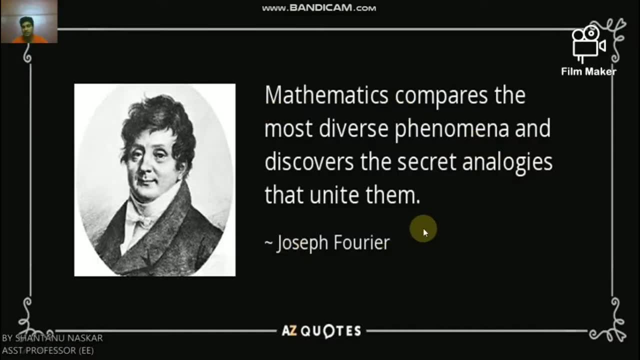 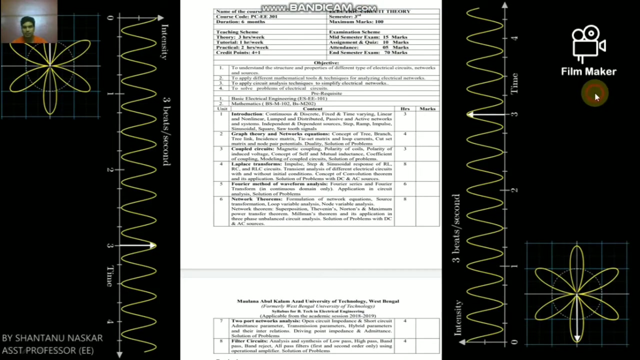 So before starting this lecture, I want to share with you something that was told by Joseph Fourier. who invent Fourier series and transform that mathematics compares the most diverse phenomena and discover the secret analogies that unite them. Now let us talk about your syllabus. So name of the course is electric circuit theory. 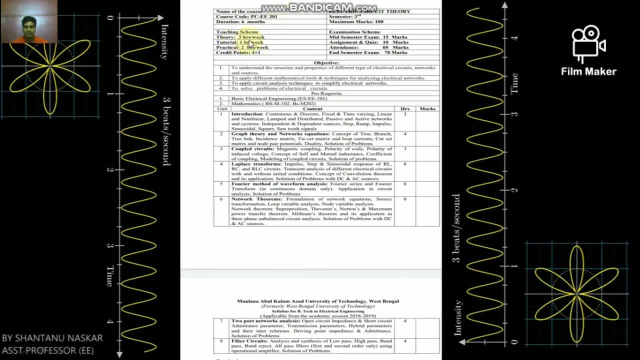 Course code PCW301 and teaching scheme: 3 hours per lecture, 3 hours per week lecture And this is the theory class and tutorial 1 hour per week and practical 2 hours per week And credit point 4 plus 1.. So about this objective and this content I have already discussed. 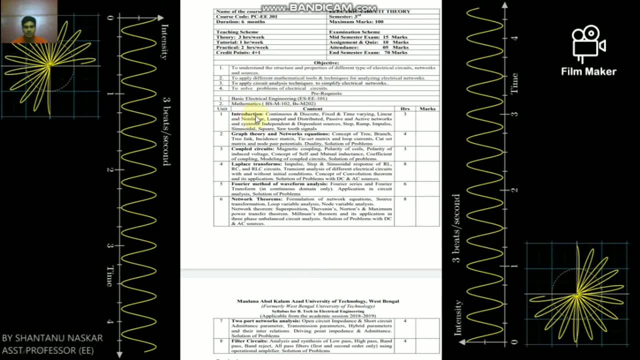 in my previous classes, So I have already completed introduction portion: graph theory, coupled circuit, Laplace transform, network theorem, two-port network analysis and filter circuit. So only left is Fourier method, away from analysis, where I will discuss about Fourier series and Fourier transform and application in circuit analysis. 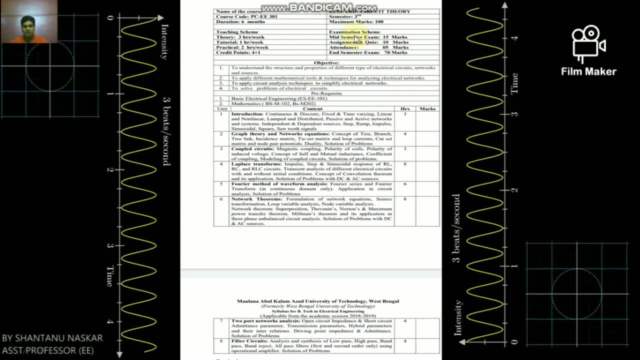 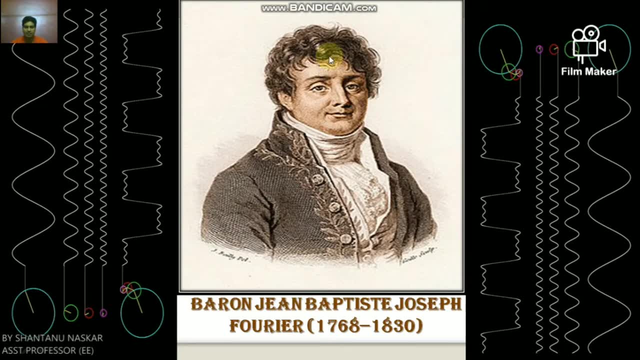 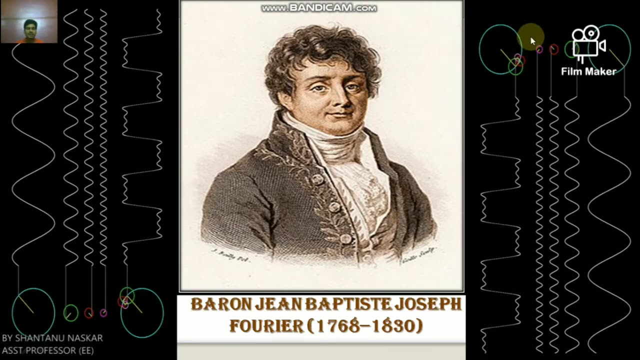 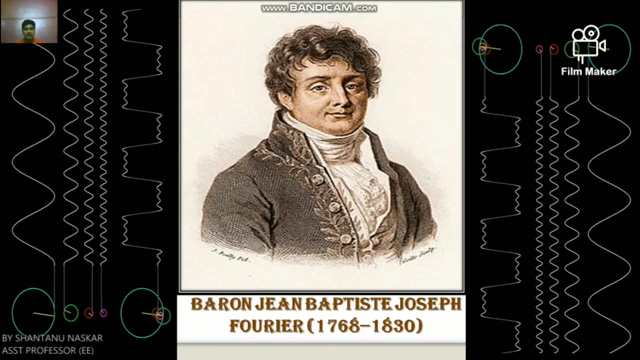 So let us start. So who is Baron Jean-Baptiste Joseph Fourier? In 1887, the French mathematician Joseph Fourier submitted a paper to the Academy of Science in Paris. In it, he presented a mathematical description of problem involving heat conduction. 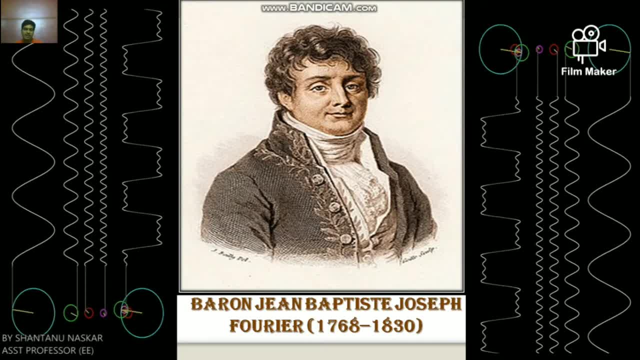 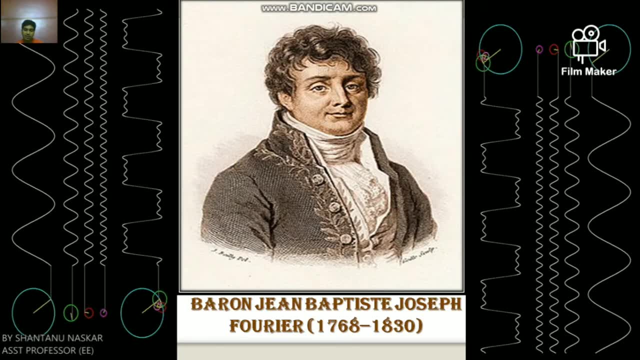 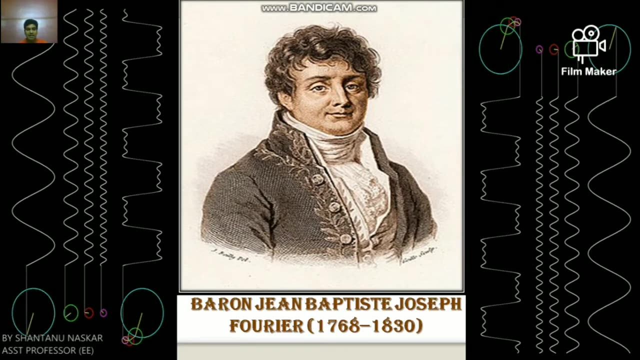 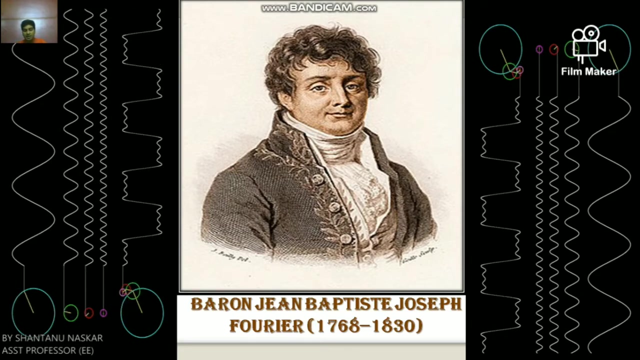 Although the paper was at first rejected, it contains ideas that would develop into an important area of mathematics named in honor: Fourier analysis. One surprising ramification of Fourier works was that many familiar functions can be expanded in infinite series and integrals involving trigonometric functions. 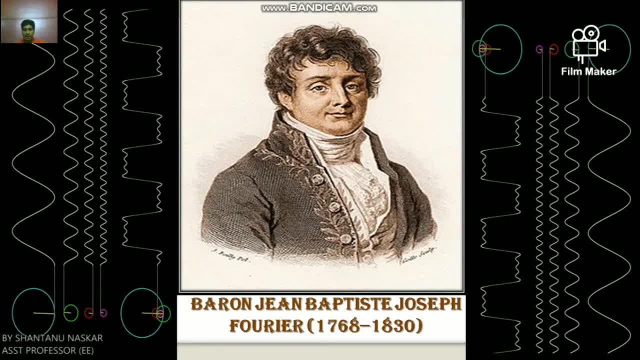 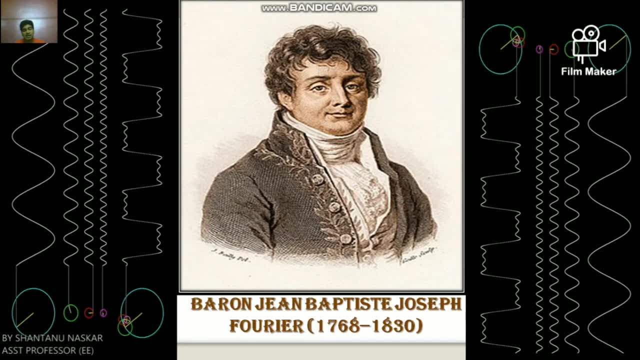 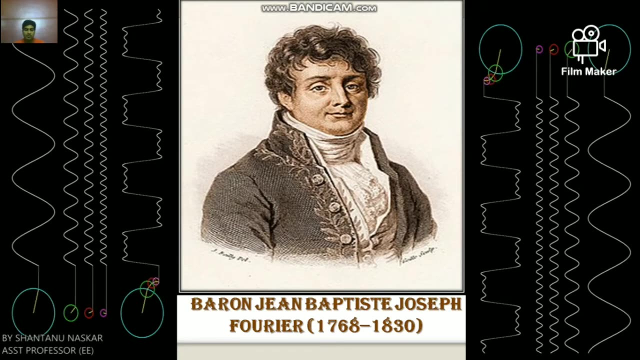 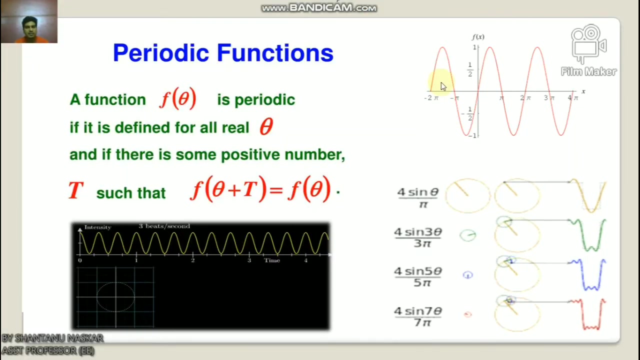 The idea today is important in modeling many phenomena in physics and engineering also. So Fourier analysis is a method for analysis of steady state response of a network subject to a periodic input. So before knowing this Fourier series and transform, you have to know what is periodic. 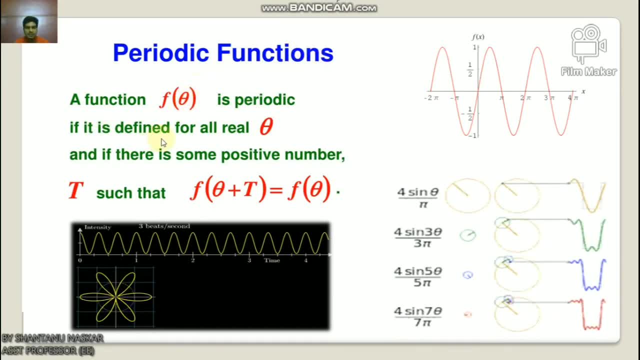 function. So function f theta is periodic input. So function f theta is periodic input If it is defined for all real theta and if there is some positive number t, such that f theta plus t equals to f theta. So let's come to the point Fourier series. 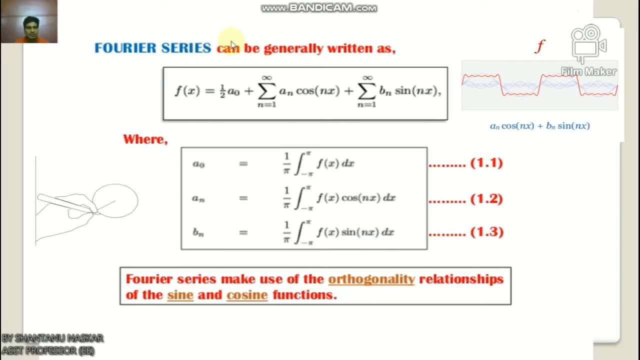 So French mathematician JBJ Fourier first started the periodic function in 1822 and published his theorem which states that any arbitrary periodic function can be replaced by an infinite series of sinusoidal of harmonic related frequencies. This infinite series is known as a Fourier series. 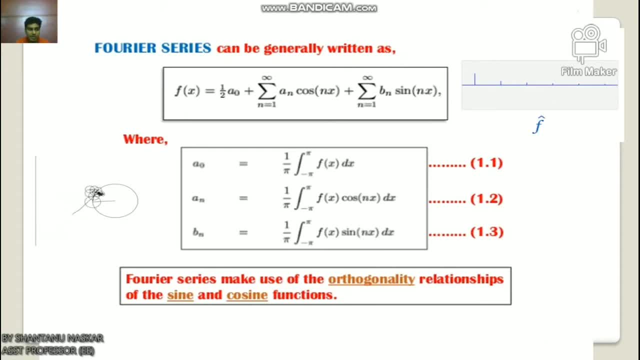 So when f is a periodic function, then Fourier series is f equals to a0 plus a1 cos x plus h2 cos x plus an cos x. Thus f is a periodic function. then Fourier series is f equals to a0 plus a1 cos x plus. 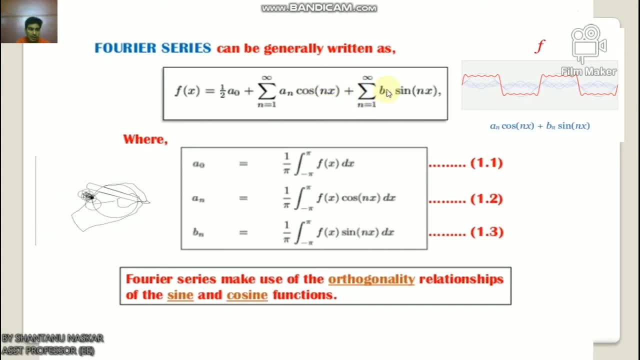 h2 cos x plus a1 sin x, And b1 sin x is, of course, b2 sin x. So these are our theories. So we need to remember that before understanding Fourier analysis, we need to know that this time the function f is going to be useful and the function is going to be used in arithmetic. 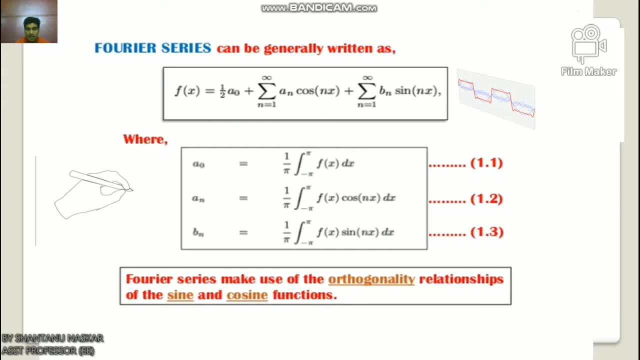 So this is what we are going to learn today: to sine 2x, B 3 sine 3x, like this: B n sine nx. so summation of all of this Fourier series can be generally written as: fx equals to half a 0 plus summation. 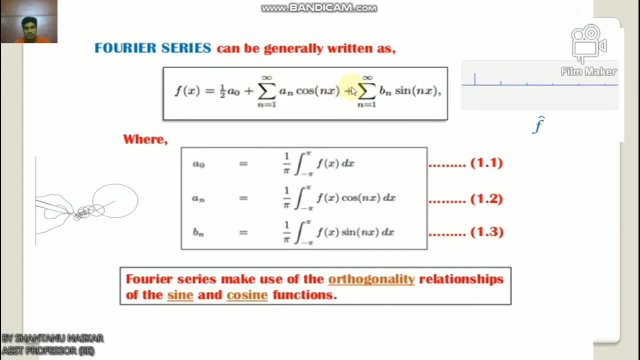 n equals to 1 to infinity n cos nx plus summation. n equals to 1 to infinity B n sine nx, where a 0 equals to 1 by Phi infinity integration minus Phi Phi, fx dx, and n equals to 1 by Phi integration minus Phi, Phi fx cos nx, dx and B n. 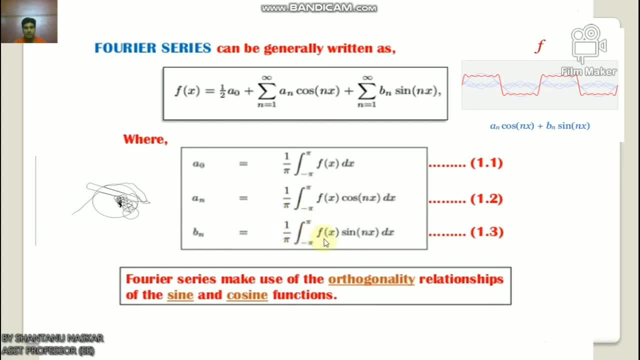 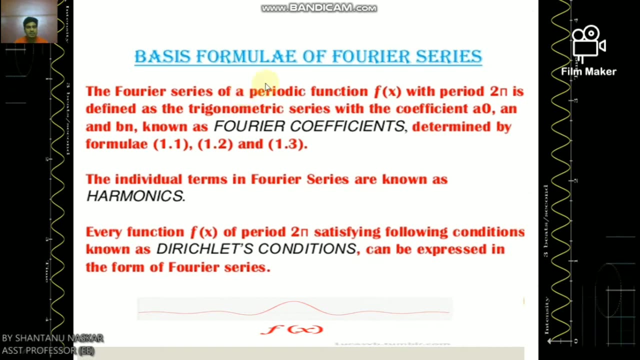 equals to 1 by Phi integration minus Phi. Phi, fx, sine, nx, dx. so Fourier series make use of orthogonal relationship of the sine and cosine function. so basics formulae of Fourier series. the Fourier series of periodic function, fx, with periodic 2. Phi is defined as the trigonometric series with the coefficient of a: 0 and B n and B n. 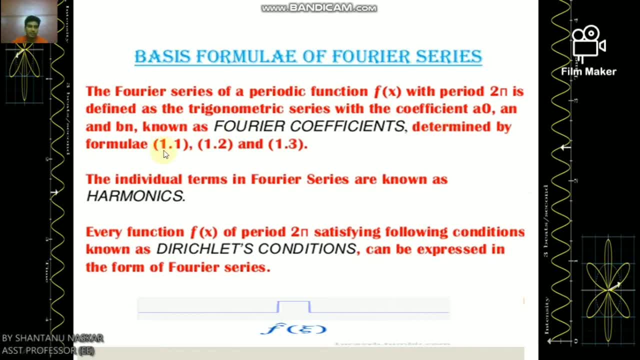 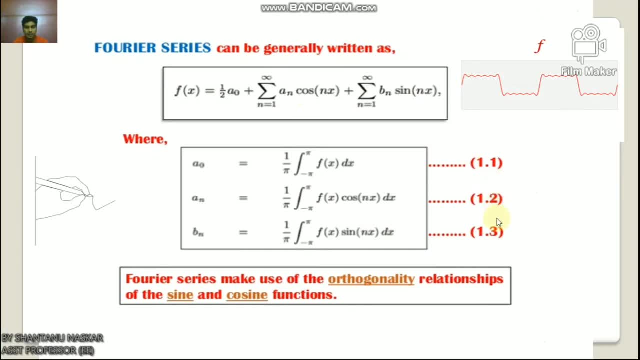 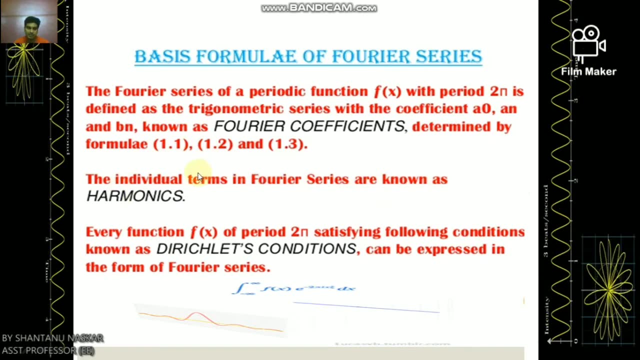 known as Fourier coefficients determined by formula 1.1, 1.2 and 1.3. took here 1.1, 1.2 and 1.3, so this individual term in Fourier series are known as harmonic. okay, so every function fx of period d, period 2. 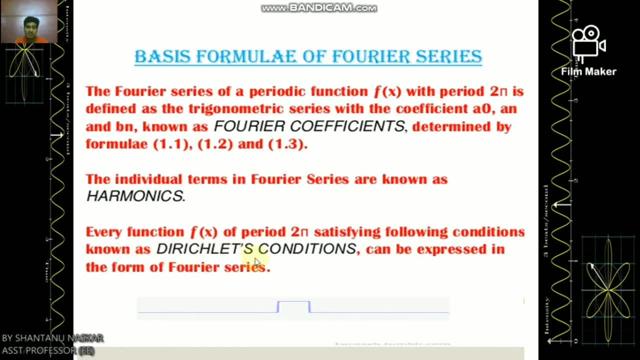 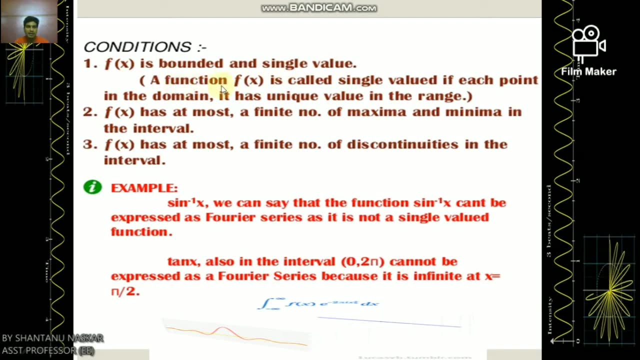 satisfy following condition known as Dirichlet condition, can be expressed in the form of Fourier series. so what is Dirichlet condition? I will discuss later. so the conditions are: fx is bounded and single value a function. fx is called single value if each point in the domain it has unique value in the range and 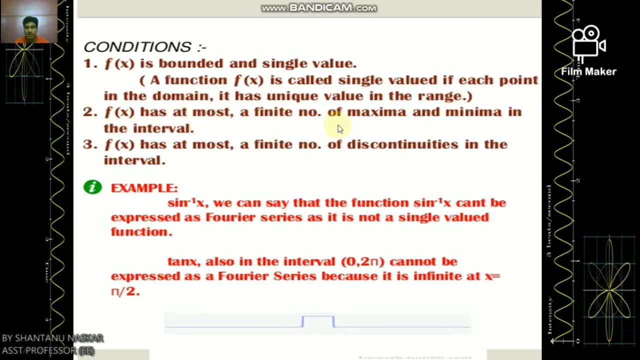 number two, fx, has at most a finite number of maximum and minima in the interval, and number three, fx, has at most a finite number of discontinuities in the interval. example, if sine inverse x, we can say that the function of sine inverse 1x. 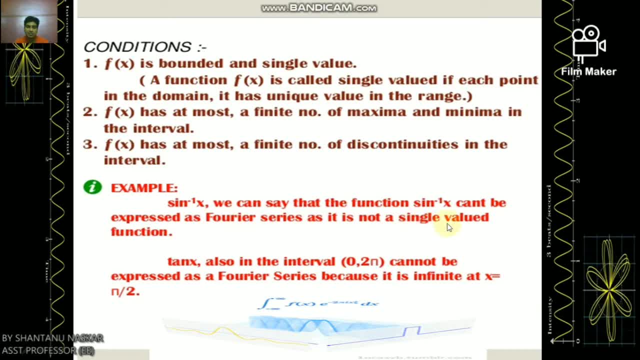 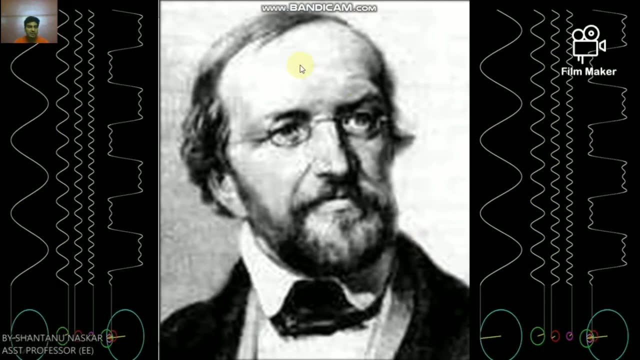 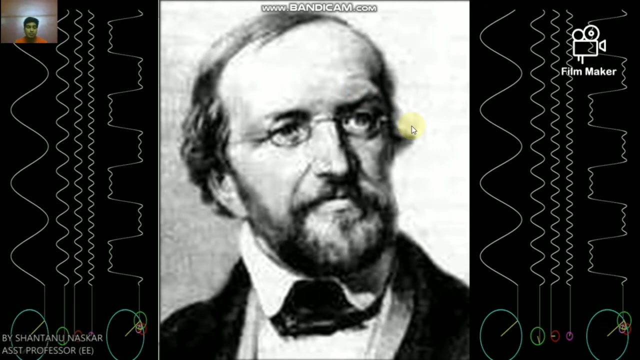 can't be expressed as Fourier series as it is not a single valued function. and tan x, also in the interval 0 to Pi, cannot be expressed as a Fourier series because it is infinite, at x equals to Pi by two. so let's talk about Dirichlet condition. so who is Dirichlet? Jonathan, Johan Peter? 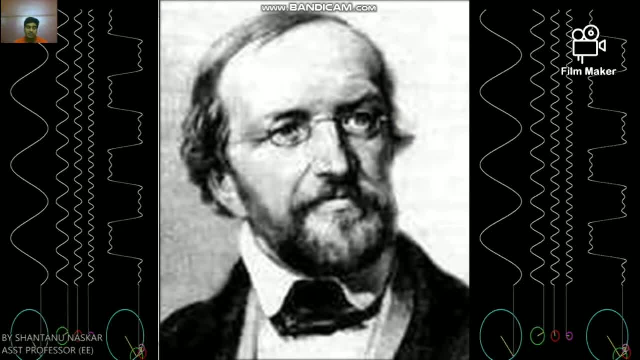 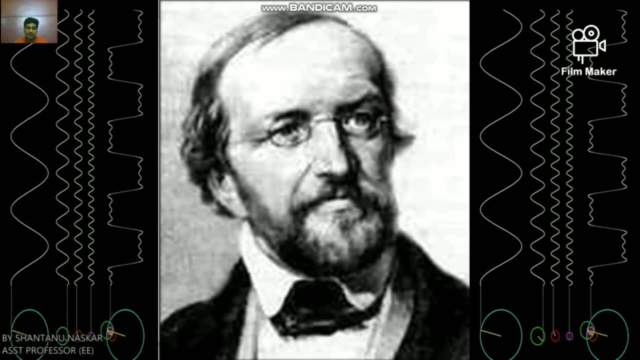 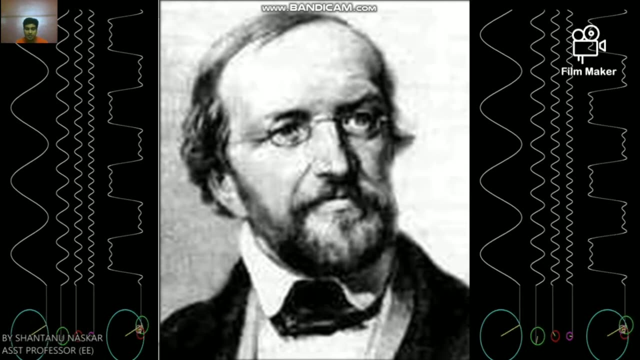 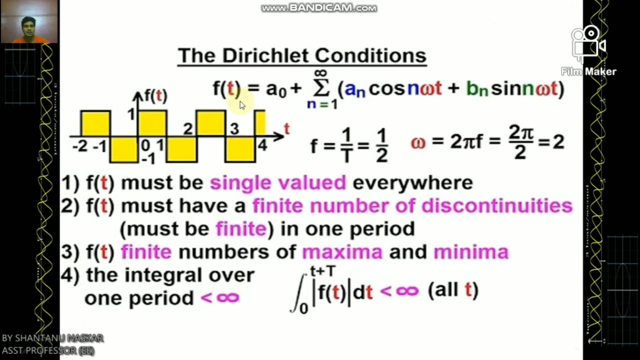 Gustav Dirichlet was a German mathematician who made deep contribution to number theory and to the theory of Fourier series and other topic in mathematical analysis. so he is created with being one of the first mathematics to give the modern formal definition of function. so what is the Dirichlet condition? same as f, t equals to a 0 plus and summation n equals to. 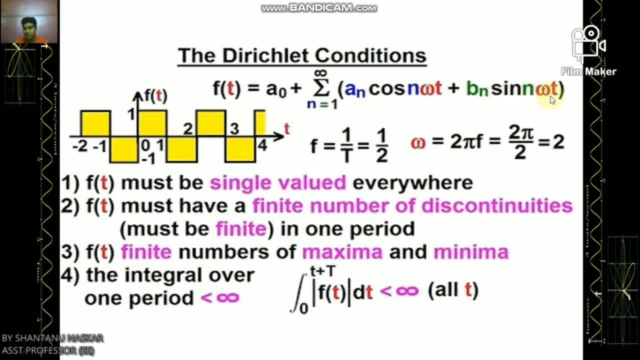 1 to infinity. a n cos n Omega t plus b n sine n Omega t. okay, so function f equals to 1 by t equals to 1 by half. omega equals to two pi f. two pi by two equals to two. so condition is one number. 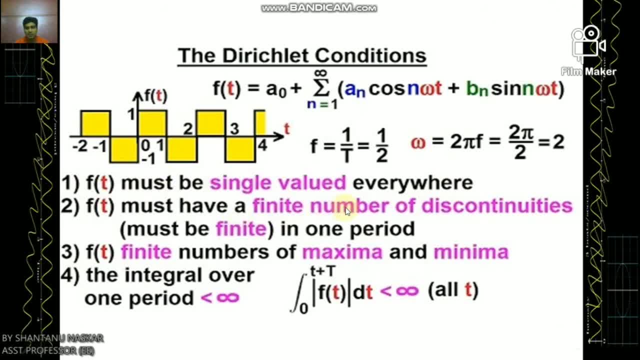 one. f? t must be single valued everywhere and f? t must have a finite number of discontinuities and must be finite in one period. number three: f, t, finite numbers of maximum and minima. number four: the integration over one period less than infinity. so condition: 0 to t plus t, f? t, dt, less. 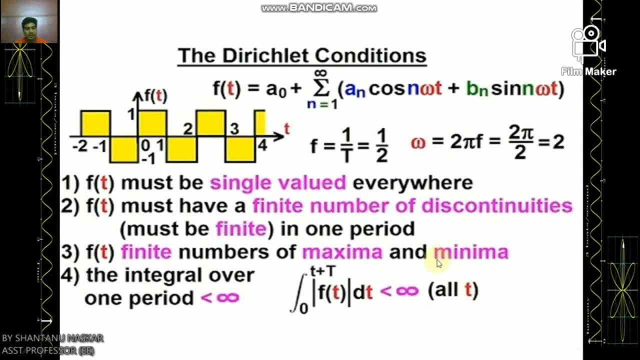 than equals to infinity for all t. so if this function represented energy which would be supplied by the source in one cycle, that means the energy in the waveform, for which cycle must be finite. so all physical waveform would of course satisfy this criteria. therefore, in practical engineering problem it is not necessary to 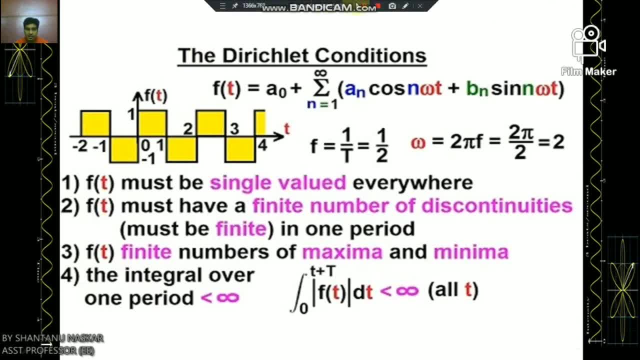 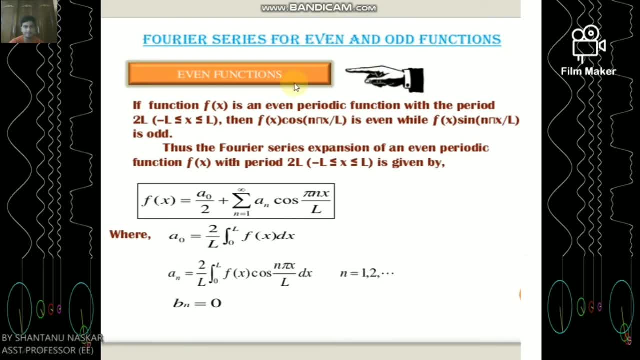 check whether a function satisfied Dirichlet condition. now let's talk about Fourier series for even an odd function, for even function. if function f is an even periodic function with video to x equals to less than equals to minus L, greater than equals to minus L and less than equals to L, 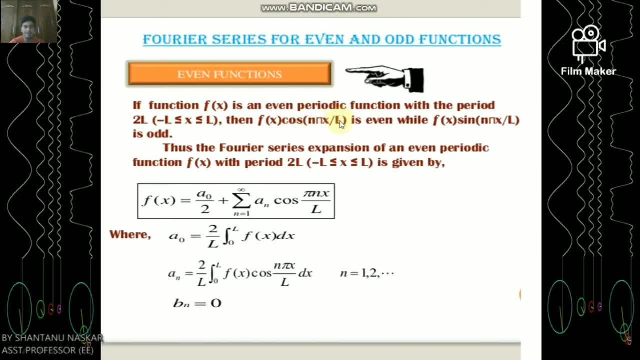 then f x cos n pi x by L is even, while f x sine n pi x by L is odd, okay, so thus the Fourier series explanation of an even periodic function: f x with video to L. when x greater than or equal to x is less than equals to minus L and less than equals to L is given by f, x equals to a 0 by 2 plus summation. 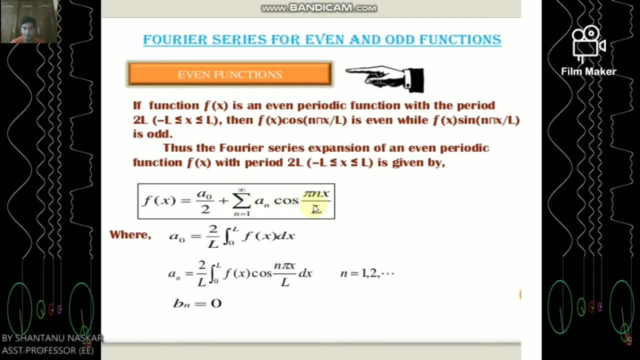 of n equals to 1 to infinity, a n, cos, pi, n, x, y, L, and where a 0 equals to 2 by L integration 0 to L, f, x, dx, and a n equals to 2 by L integration 0 to L, f, x, cos, n, pi, x by L, dx, where n equals to one, two. 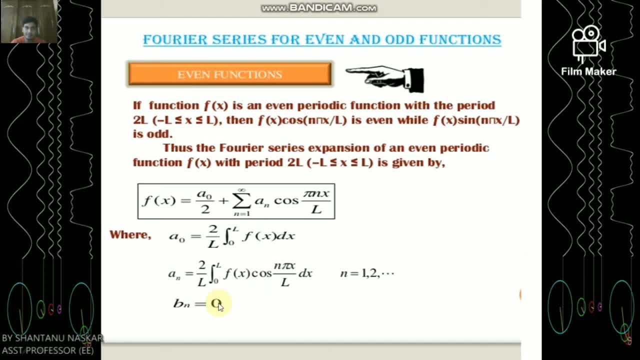 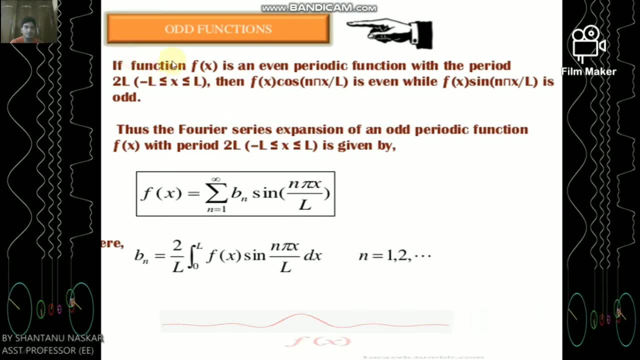 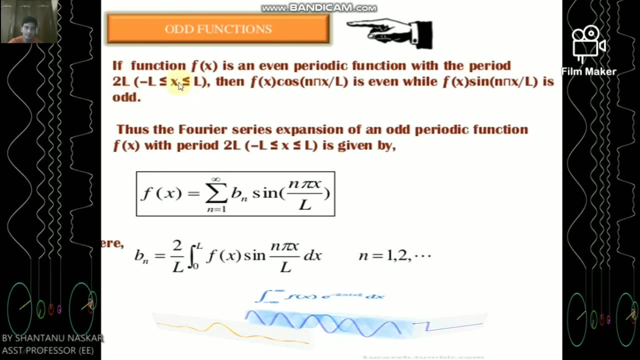 can you write that. you speak any number. you can write a function f x. because of that, the function f x is an even periodic function with the period to L, while f x rescaled because of the L integration. so these are just two important problems that you need to work. 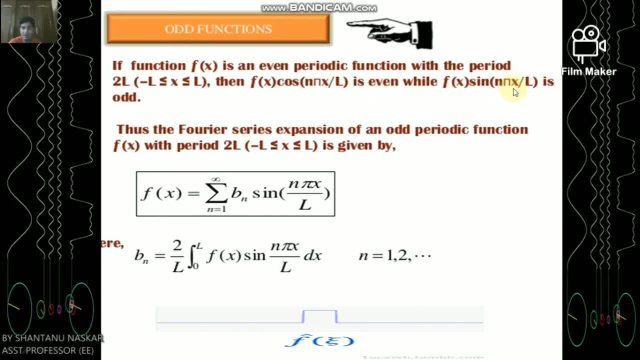 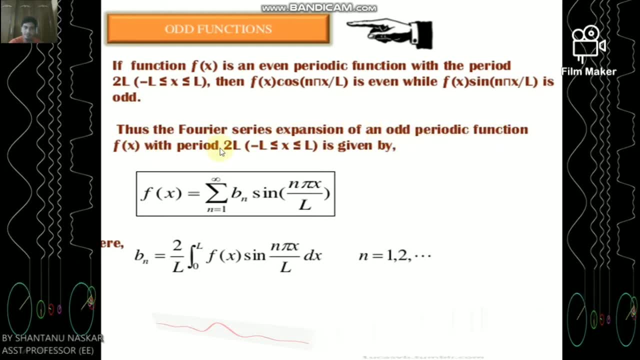 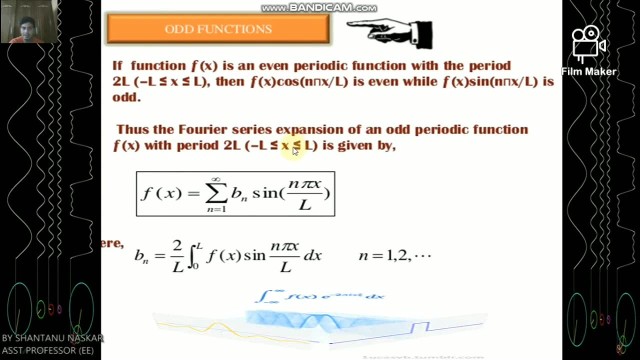 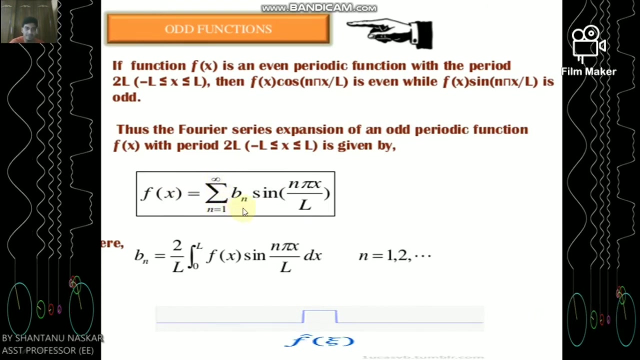 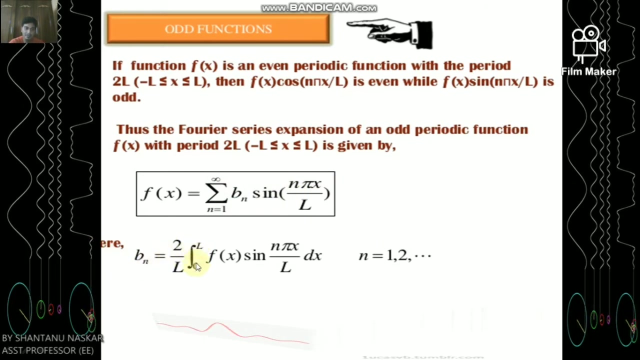 out as a tutorial. just keep this as simple as possible if you see the человеч時間. so this, Thus the Fourier series expression of an odd periodic function, fx, with period 2l. where x, greater than equals to minus l and less than equals to l, is given by fx equals to summation of n equals to 1 to infinity bn sine n phi x by l. where bn equals to 2 by l, integration 0 to l. fx sine n phi x by l, dx, y. 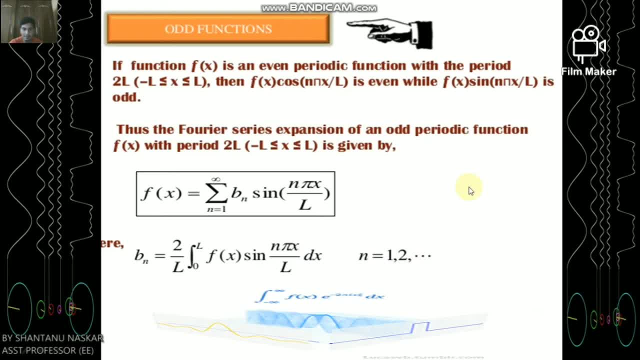 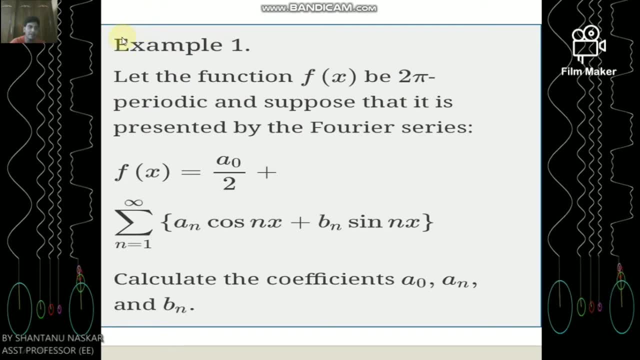 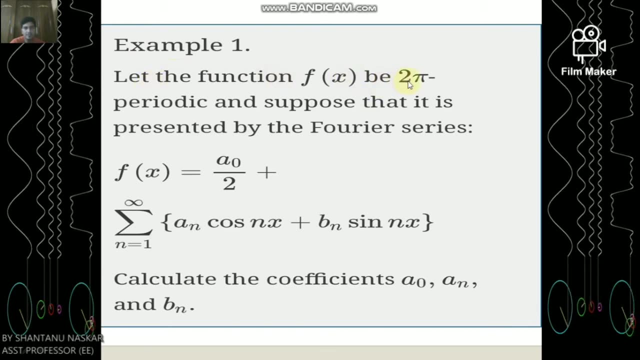 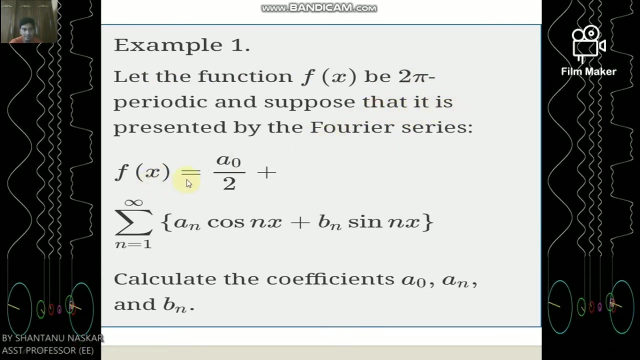 where n equals to 1, 2, 3, 4, like this. Now here is I will discuss about an example mathematics of Fourier series. So let the function fx be 2, pi periodic and suppose that it is presented by the Fourier series. fx equals to a0, y2 plus integration sum. 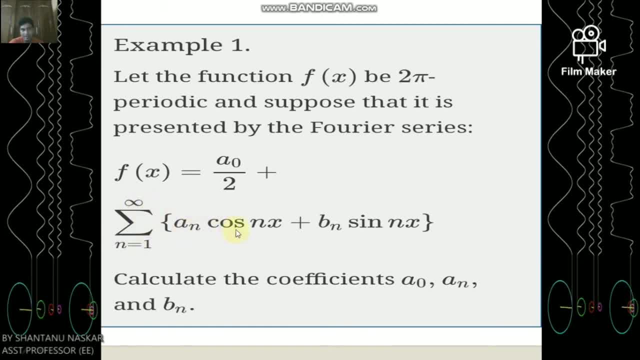 So let the function fx be 2, pi periodic and suppose that it is presented by the Fourier series. fx equals to a0, y2 plus integration sum and n equals to n. equals to 1 to infinity of a, n, cos, n, x plus b, n, sine, n, x and calc. now calculate. 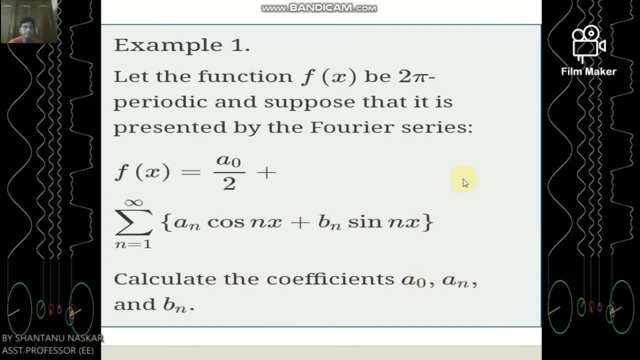 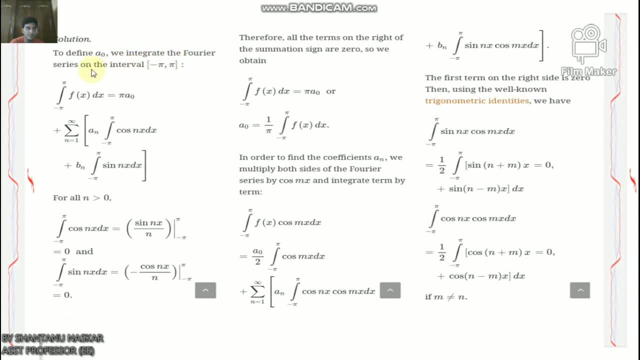 the coefficient a, 0, a, n and b? n. so let's talk about the solution to define a: 0. integrate the Fourier series on interval of minus pi to pi. so integration minus pi to pi, fx dx equals to pi a 0 plus summation of n equals to 1 to infinity of a? n. integration cos n x dx interval is minus pi to. 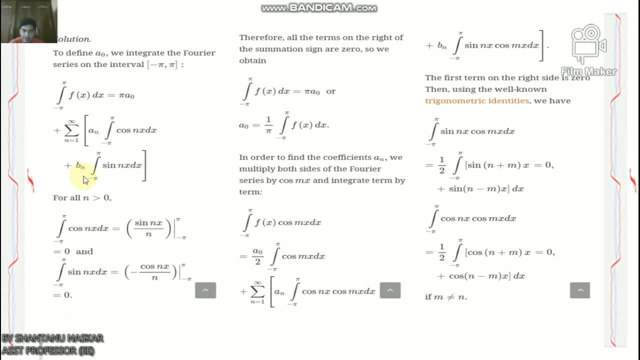 pi plus b? n. integration minus pi to pi sine n x dx for all n greater than g. now, integration cos n x dx. interval minus pi to pi equals to sine n x by n okay, which is equals to 0, and this is the interval. and sine n x dx to integration sine n x dx. interval minus pi to pi. 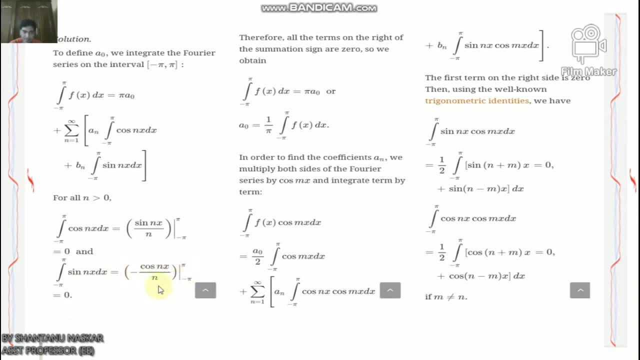 equals to minus cos n x by n- this is the interval- equals to 0. therefore all the term on the right on the summation sign are 0. so we obtain: integration minus pi to pi fx dx equals to pi a 0, or a 0 equals to 1 by pi integration fx dx. so in order to find the coefficient n a n, we multiply: 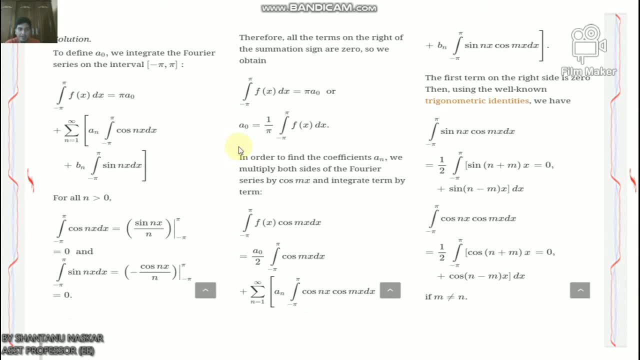 both both sides of the Fourier series by cos m- x and integrate term by term, which is: integration minus pi to pi fx. cos m x- dx equals to a 0 by 2. integration minus pi to pi, cos m x, dx plus summation of n equals to 1 to infinity within bracket n. integration minus pi to pi, cos n x, cos. 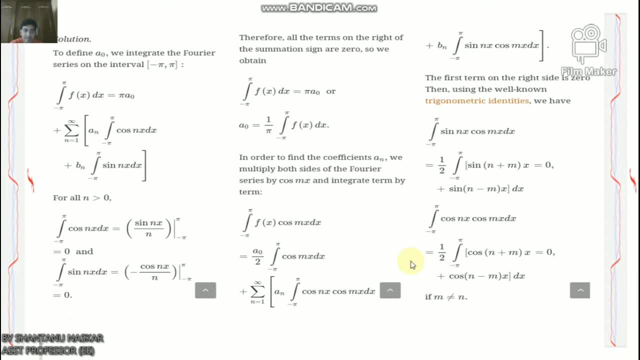 m x dx plus b n. integration minus pi to pi sine n x, cos m x, dx. so the first term of the right side is 0. then, using the well-known trigonometric identification, we have integration minus pi to pi sine n x, cos m x, dx. 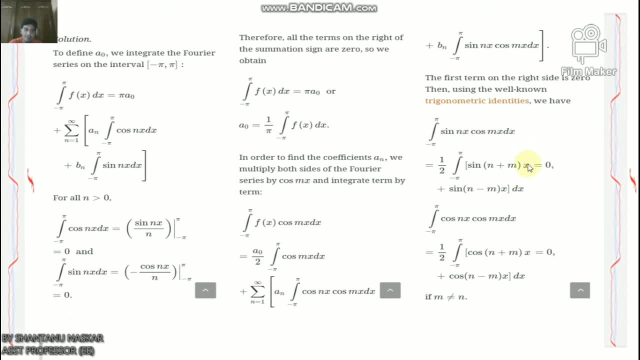 equals to half integration minus pi to pi within bracket. sine n plus n m. n plus m x equals to 0, plus sine n minus m x dx and integration cos n x, cos m x dx equals to half integration minus pi to pi. cos n plus m x equals to 0. 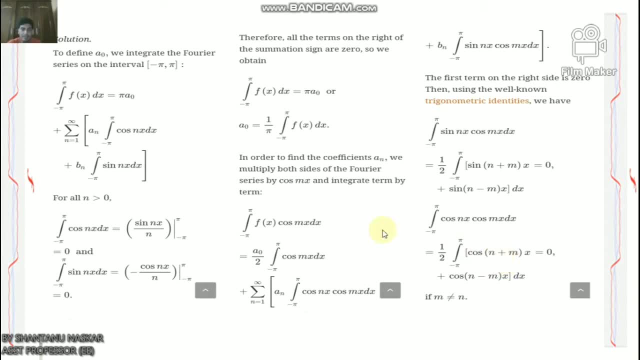 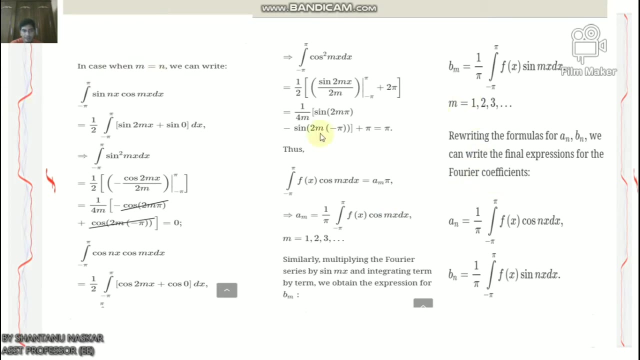 plus cos n minus m x dx. so if m not equals to m, then in case when, so before that condition in if m not equals to n, in case of m equals to n, we can write: integration minus pi to pi sine n x. cos m x dx equals to half integration. minus pi to pi sine 2 m x plus sine 0 dx equals to integration minus. 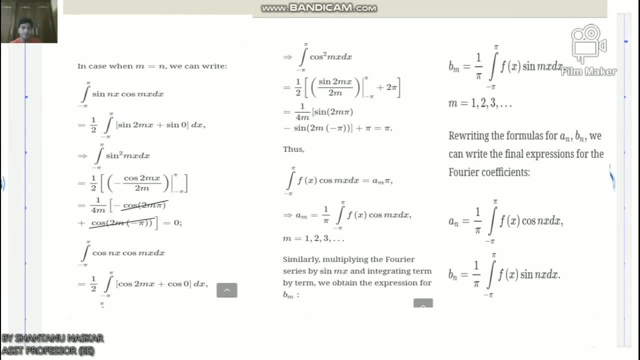 sine square m x dx equals to half cos minus cos 2 m x by 2 m. so this is the interval pi to minus minus y to phi, which is equal to 1 by 4 m within bracket. minus cos 2 m pi, plus cos 2 m phi equals to: 0. so we can write: integration minus pi to pi sine 2 m x plus sine 0, dx equals to half integration minus phi to pi sine 2 m x plus ou y m plus. interrupting sine 2 ayuda and e value will be less than pi. 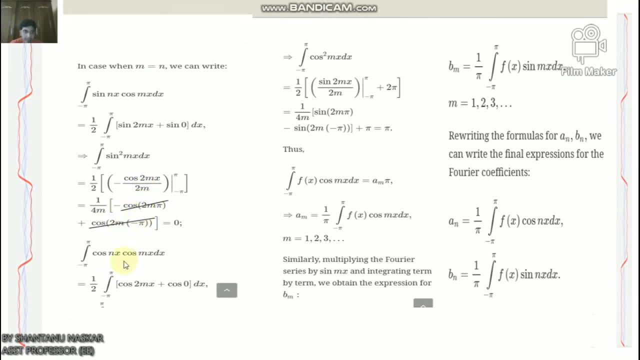 and w this two things. we can write: integration minus pi to pi. cos n, x, cos m x dx equals to half integration. minus filling flaco skew x equals to integration hapsine to waste them in collaboration phase. so for example, in m sine 2 m y and minus 2 m within bracket. minus pi plus pi equals to pi. thus 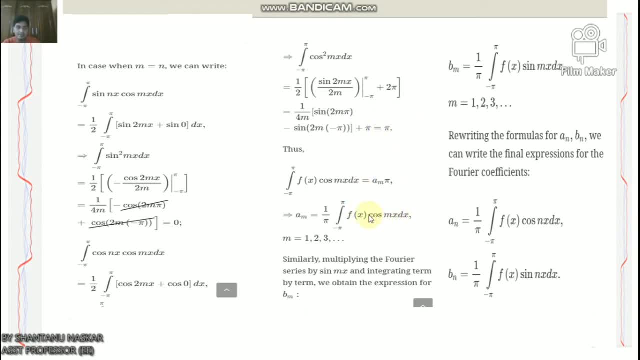 integration minus pi to pi: fx cos, mx, dx equals to a m pi and a m equals to 1 by 5. integration minus pi to pi: fx cos, mx, dx, where m equals to 1, 2, 3. like this, similarly, multiplying the Fourier series by sine mx and integrating term by term, we obtain the expression for bm and bm equals to 1. 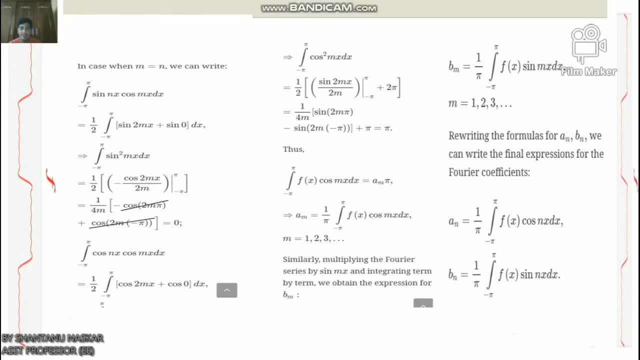 by pi integration minus pi to pi, fx sine mx, dx, where m equals to 1, 2, 3, like this, and rewriting the formula for a, n, b, n, we can write the final expression: you, for the Fourier coefficient, which is a, n equals to 1 by pi integration minus pi to pi, fx cos mx. 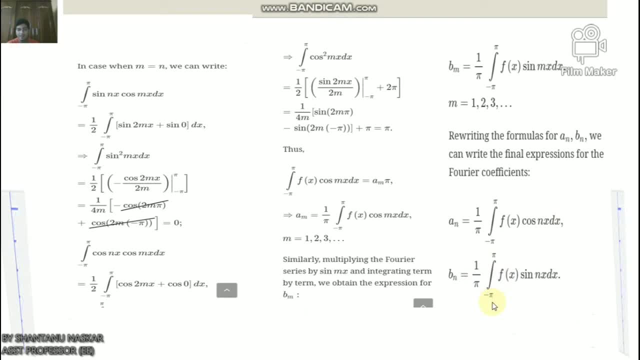 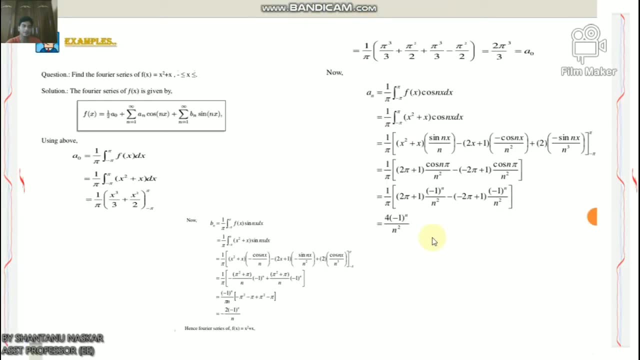 dx and bm equals to 1 by pi integration minus pi to pi fx sine mx dx. let's talk about another example. question is: find the Fourier series of fx equals to x square plus x. so solution is: the Fourier series of fx is given by this equation. 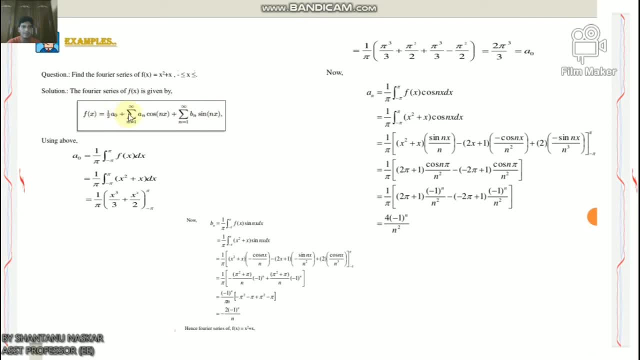 you all know the equation: fx equals to half a zero plus summation of n equals to 1 to infinity v n, coshh, nx, plus summation of n equals to 1 to infinity b n sine nx, nx. so using this above equation, we can get the value of a0, which is equals to 1, by pi integration. 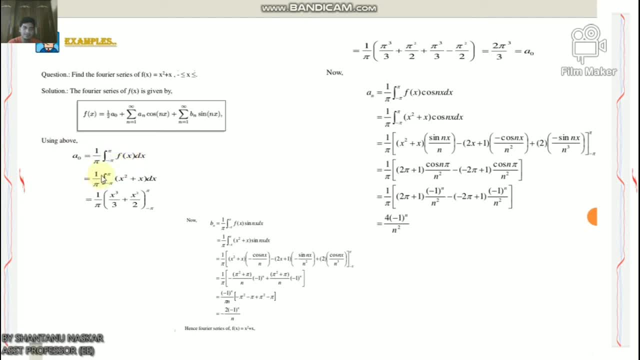 minus pi to pi, f s DX and equals to 1 by pi. integration minus pi to 5x square x plus dS. so by integrating this thing we can conclude the value 1 by pi. if you have 1 by pi in the random id-yating string we can add equal to one by pi integration minus pi to into 5 xs, ys plus dS. so by integrating this thing we can compute the value one. 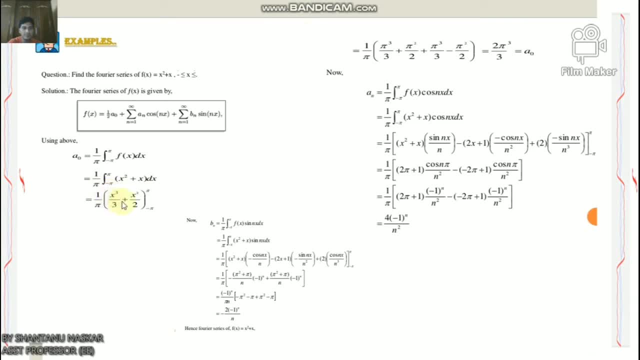 conclude, the value 1 by pi equals to x cube by 3 plus x square by 2. interval is minus pi to pi, so the value is 1 by pi and within bracket, pi cube minus by 3 plus pi square by 2 and plus. 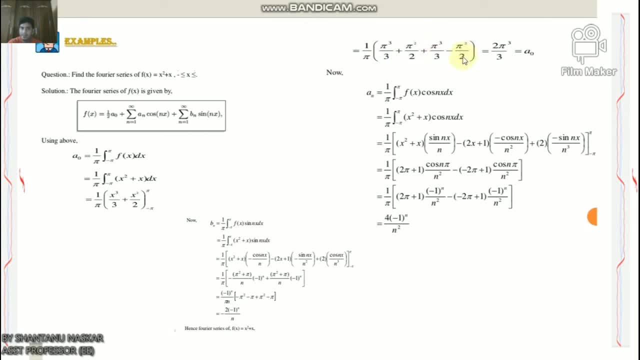 pi cube plus by 3, minus pi square by 2, so the whole value is a 0 equals to pi cube by 3. now for n: n equals to 1 by pi. integration minus pi to pi, fx, cos, nx, dx, which is equals to 1 by pi. 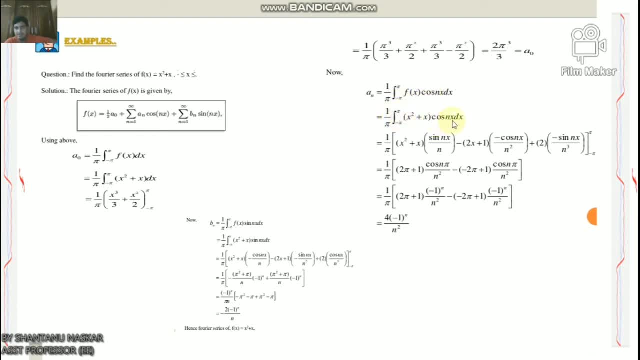 integration minus pi to pi, x square x cos nx, dx, so which is equals to 1 by pi within bracket x square x sine nx by n minus 2x plus 1 within bracket minus cos nx by n square plus 2 minus sine nx by n cube, and the whole is an interval of minus pi to pi. so concluding this: 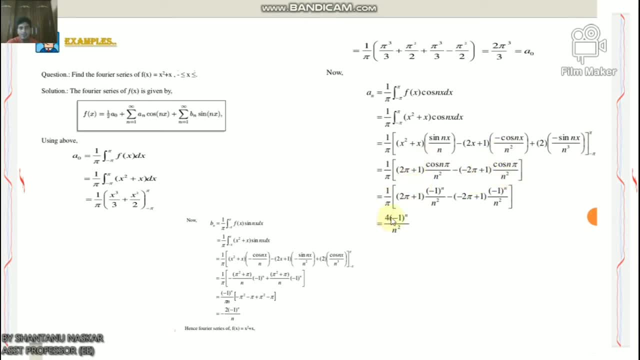 concluding this value, we can get a value is 4 minus 1 to the power n by n square, and for bn equals to 1 by pi integration minus pi to pi fx sine nx dx equals to 1 by pi integration minus pi to pi x square x sine x dx, and which is equals to 1 by pi x square x minus cos nx by n minus 2x. 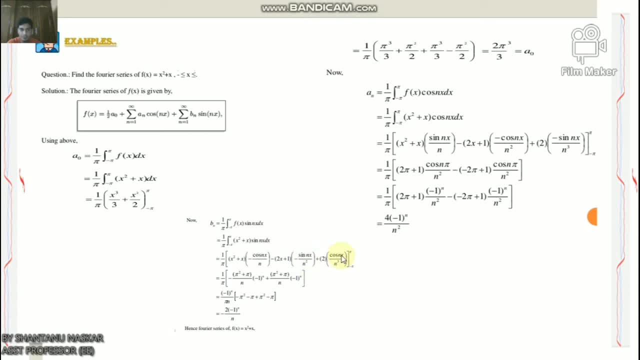 plus 1, minus sine, nx by n square plus 2, cos nx by n cube, and whole thing is in interval of minus pi to pi. so by concluding this value we can get which is equals to minus 2, minus 1 to the power n by n. so hence, Fourier series of fx, equals to x square plus x is this. this is the. 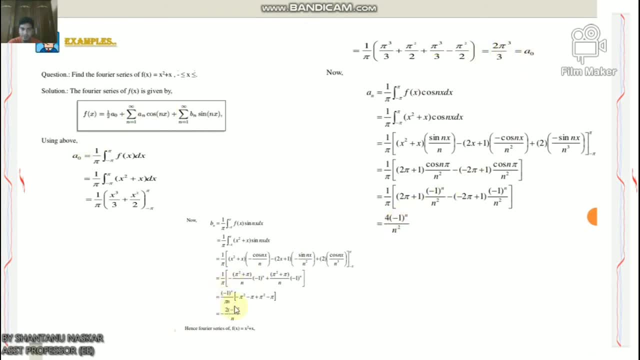 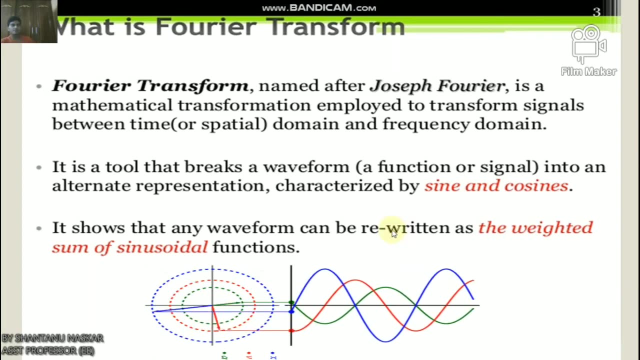 value of a: 0, this is the value of n and this is the value of bn. now comes to the Fourier transform. so what is Fourier transform? Fourier transform- name after Joseph Fourier- is a mathematical, is a mathematical transformation employed to transform signal between time or spatial domain and frequency. 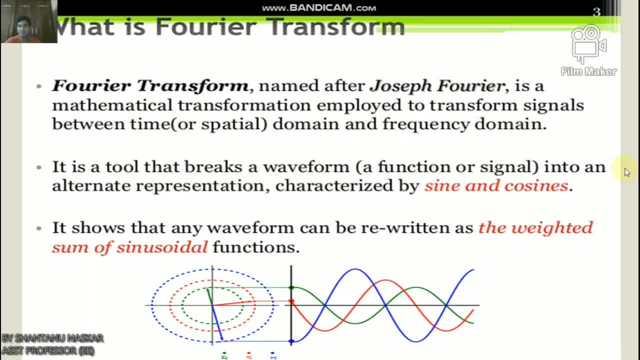 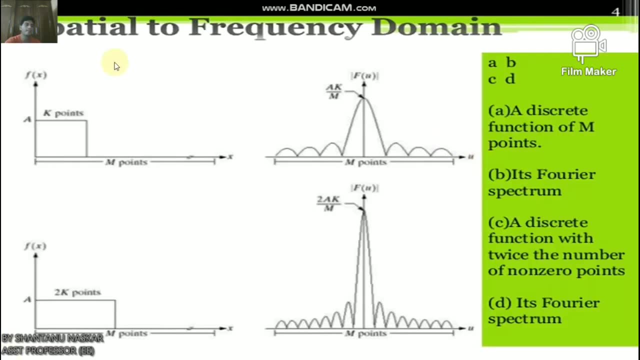 domain. so it is a tool that breaks away from a function or signal into an alternative representation characteristics by sine and cosine. it shows that any waveform can be rewritten as the weighted sum of the sinusoidal function. so now we will discuss spatial two frequency domain. so look at this four picture: a is the diskit function of N points and B its Fourier. 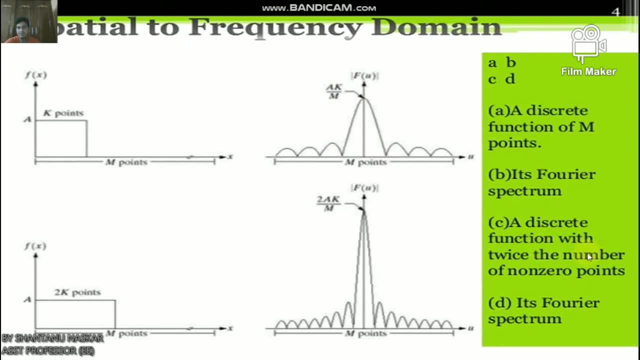 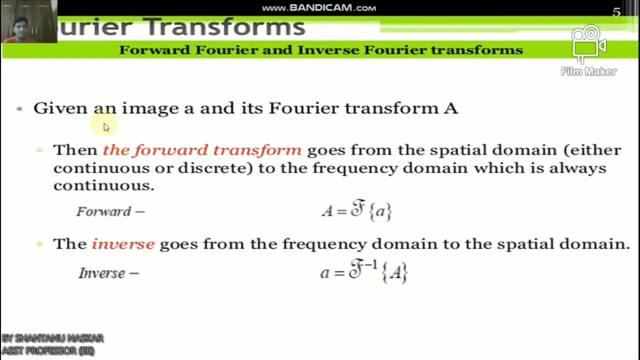 factor, and C the diskit function, with twice a number of nonzero point, and these each Fourier 's vector. so just for example Now Fourier transform, so forward Fourier and inverse Fourier transform. so given an image a and its Fourier transform is caps a, so then the forward transform goes from the spatial domain either. 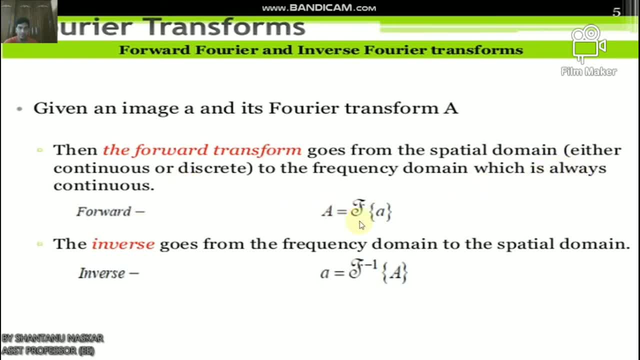 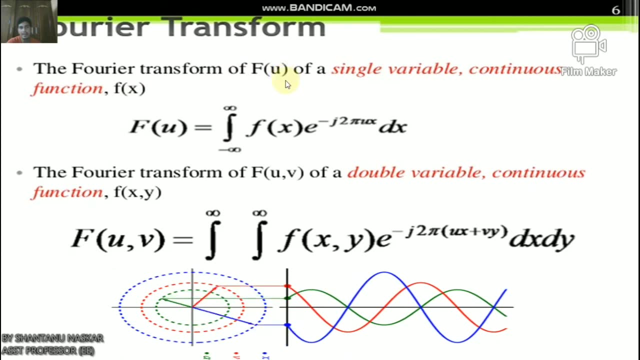 continuous or discrete, to the frequency domain, which is always forward. so a Fourier a and the inverse goes from the frequency domain to the spatial domain. inverse small a equals to Fourier inverse caps. now the Fourier transform of, if you have a single variable, continues, cut and a continuous function, F, X. now if you equals to integration minus infinity to infinity. 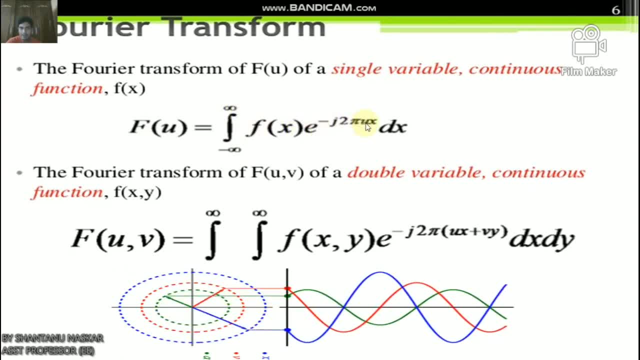 plus infinity, F? X, e to the power minus j, 2, pi? u, X, T, X. and the Fourier transform of f? u be of double variable continuous function of x, y. now F? U, B equals to integration, the infinitive integration. f x, y e to the power minus j, 2 phi u, x, plus v, y. 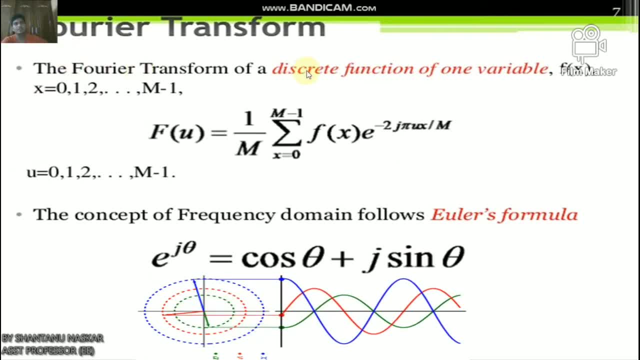 dx dy. now the Fourier transform of a discrete function of one variable: f x, x equals to 0, 1, 2, m minus 1, and if u equals to 1 by m summation, x equals to 0, m minus 1, f x, e to the power minus. 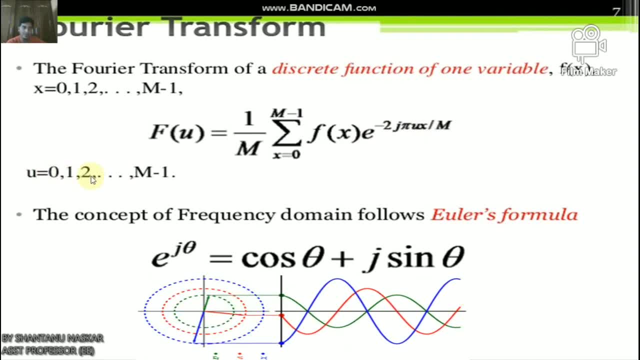 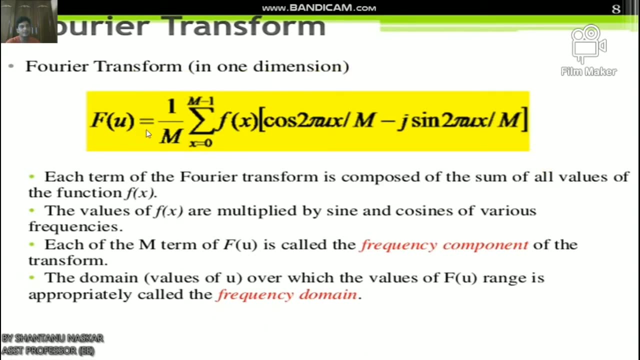 j phi u x by m. where u equals to 0, 1, 2, 2 m minus 1 and the concept of frequency domain follows the Euler's formula, which is: e to the power, j theta equals to cos theta plus j sin theta, now Fourier transform in one dimension. so f? u equals to 1 by m. summation x equals to 0 m. 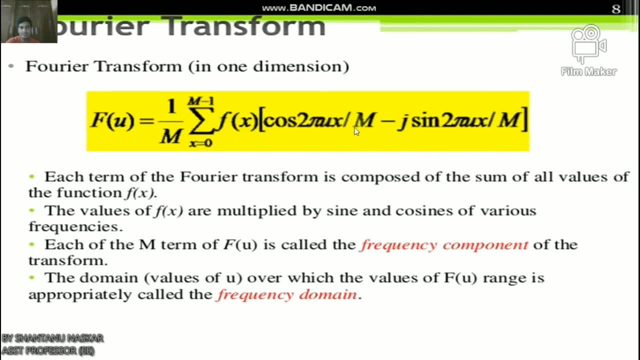 minus 1 f x, cos 2 phi u x by m, minus j sin 2 phi u x by m. so each 다음에 the Fourier transform is composed of the sum of all values of the function fx, and the values of fx are multiplied by sine and cosine of various, so each of them term of fu, is called frequency. 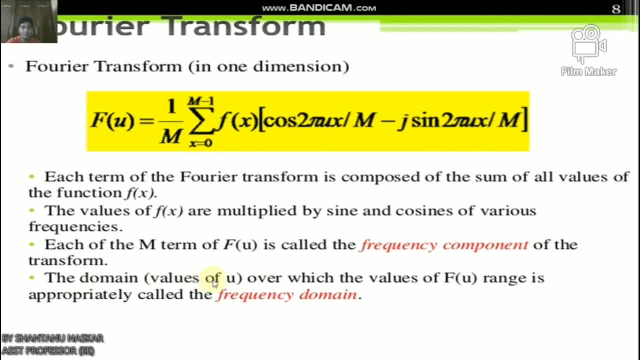 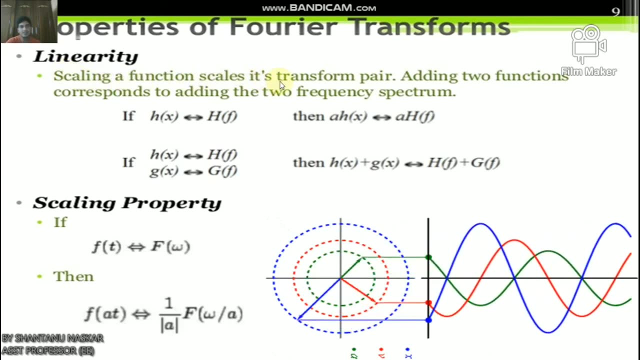 component of the transform and the domain values of u, over which the values of f? u range is appropriately called the frequency top. now properties of Fourier transform. so first is linearity, the scaling of function. scale its transform pair, adding two function corresponding to adding the two frequencies. right, look at this linearity function. 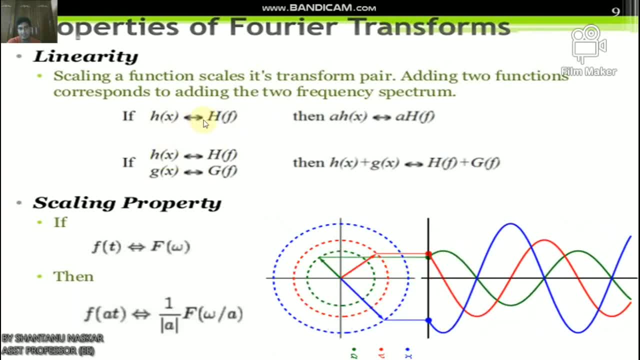 okay, hx, hf. if hx, hf and then hx, hf, gx, agf, then a hx equals to a hf, hx plus gx, which is hf plus g. so scaling property: if f t equals to f omega, then f at equals to 1 by a, f, omega by a. 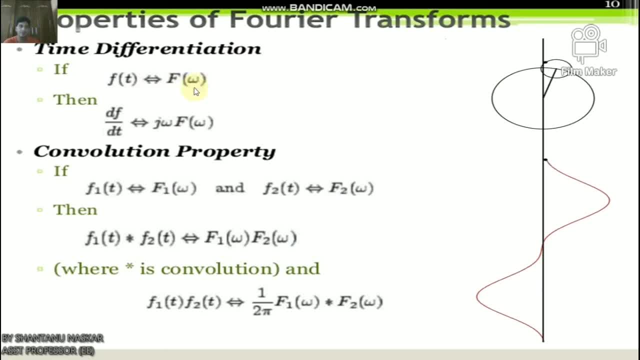 now time differentiation: if f t is 2 f omega, then d f by dt equals to j omega, f. so convolution property. if f 1 t goes to f 1 omega and f 2 t goes to f 2 omega, then f 1 convolution, f 2 t, f 1 t convolution, f 2 t equals to f 1 omega, f 2 omega, where: 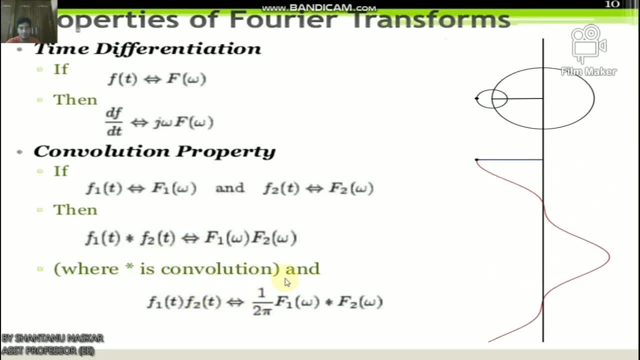 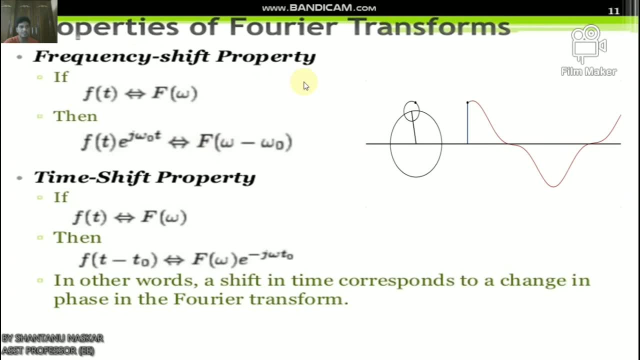 this sine is convolution, and f 1, t, f 2, three equals to 1 by 2 phi. f 1, omega, convolution, f 2, omega. now frequency shift property: if f t equals to f omega, then f t e to the power j omega 0 t equals to f omega minus omega j. 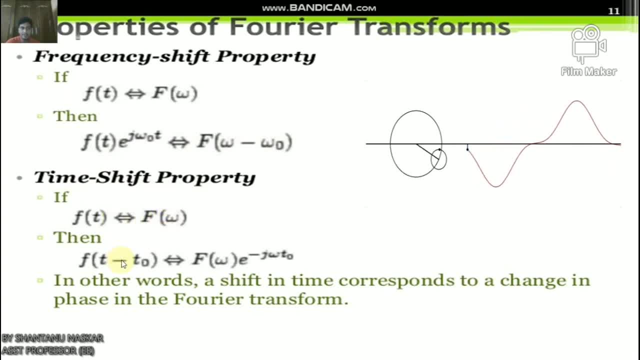 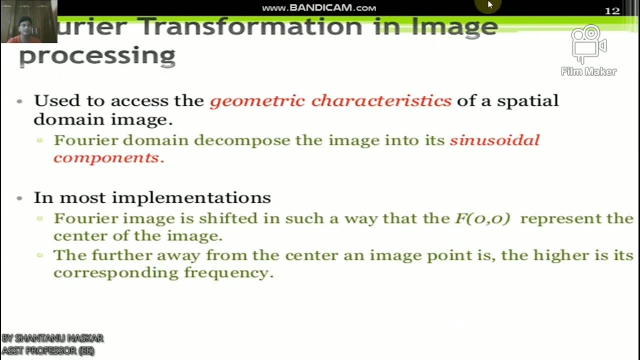 time shift property. if ft equals to f omega, then f t minus t 0 equals to f omega 0 minus j omega t was a shift in time correspondence to a change in phase in the Fourier transform, so Fourier transformation in image processing. so is used to access the. 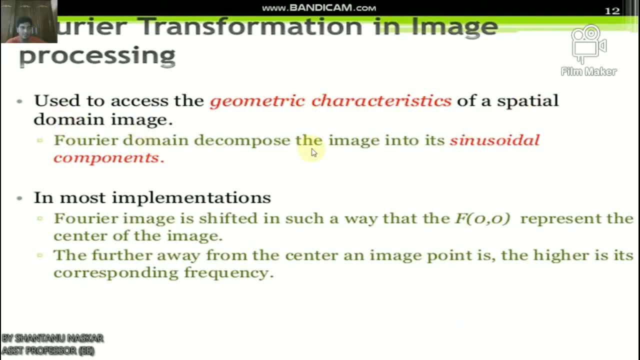 geometric characteristics of a spatial domain. image Fourier domain decompose the image into sinusoidal component. in most implementation, Fourier image is shifted in such a way that the f00 represent the center of the image. the further away from the center and image point is, the higher- is it corresponding frequency? now? 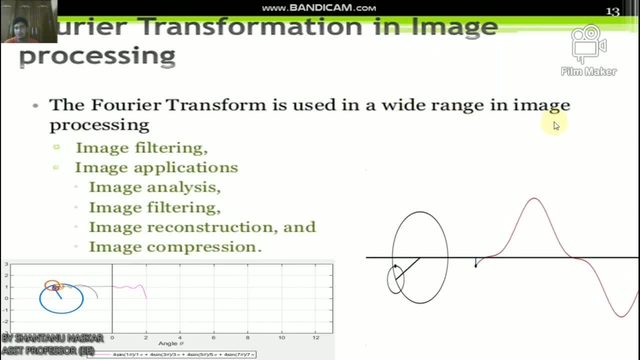 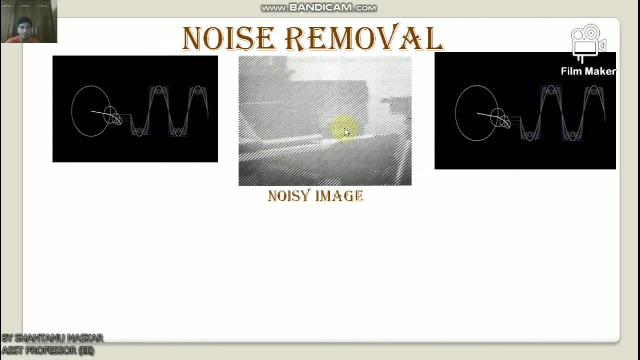 Fourier transforming image processing. next, the Fourier transform is used in a wide range in image processing, which is it for image filtering, image application, image analysis, image filtering, image reconstruction and image compression. so here is a picture with noisy noise. the image is a picture of noisy image. look.